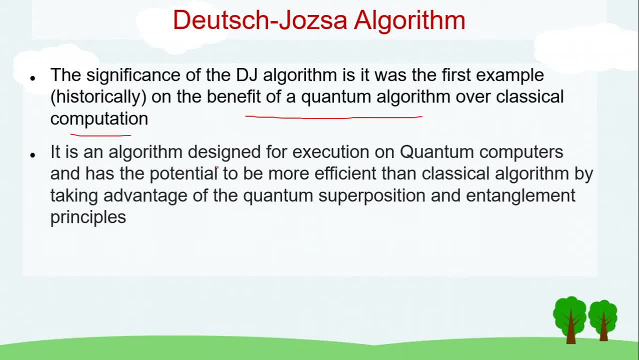 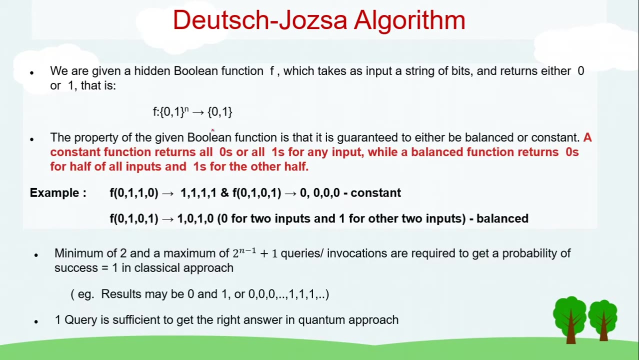 over a classical computation and it's an algorithm designed for execution on quantum computers and has the potential to be more efficient than classical algorithm by taking advantage of quantum computers properties, the superposition and entanglement. Okay, looks great. let's see how it works. What it does first, we'll understand. So this algorithm works on a Boolean function, so 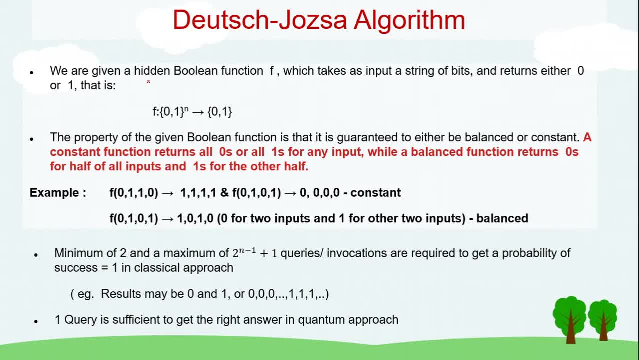 suppose we are given a hidden Boolean function, meaning a black box. we don't know what does it contain? It takes input, a string of inputs like 0, 1, 1, 0, like that, and returns either 0 or 1 for every input. Okay, so it's expressed like this: Again to let's try to. 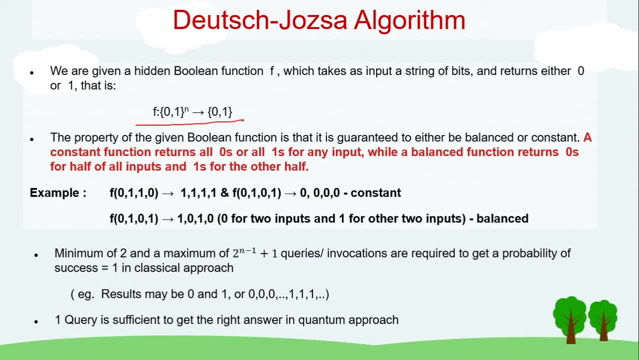 understand it in a better way. and this Boolean function has got a special property. So what is that property that it is guaranteed to be? either be balanced or constant. So what is a constant function? A constant function returns all zeros or all ones for any given input. I mean whatever. 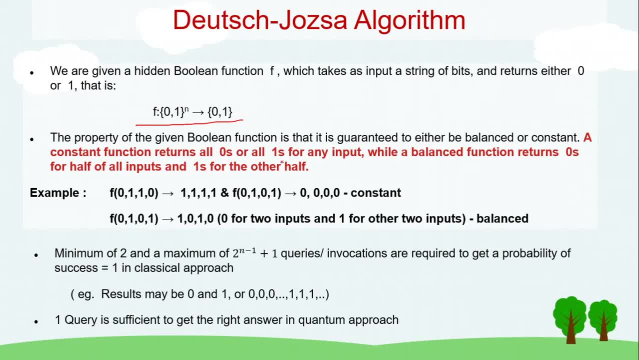 the string we have. it will give every time zeros or every times ones, So it's a constant function. Now, it is a constant function, but it also contains a function for any given value. So every time you one, while a balanced function returns zeros for half of in all inputs and one for remaining half. 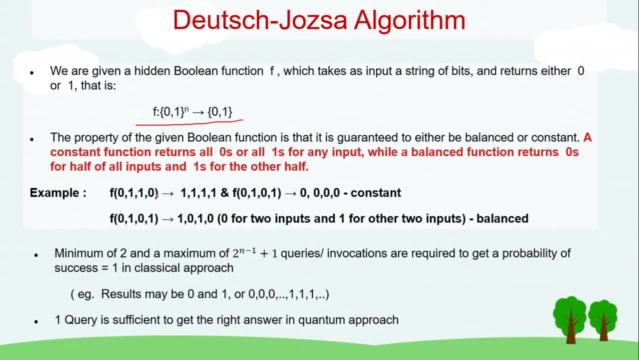 is that clear? so maybe with a number we will try to understand. suppose we argue. i mean we give the input like 0, 1, 1, 0 to the function. it may return all ones or all zeros, then it's called a constant function instead. if it returns like this, that means twice zeros and twice one, then it's a. 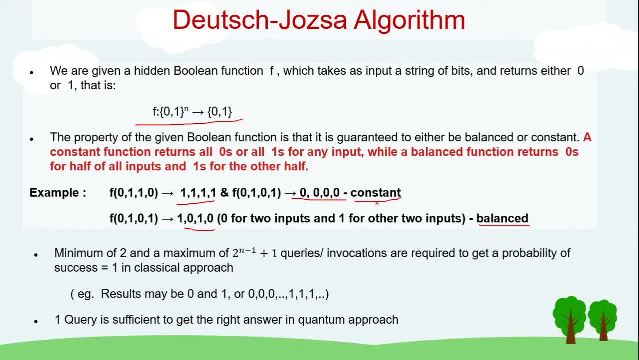 balanced function. now our job here is to find out: the given hidden boolean function is a constant or balanced one. so we need to find out. so how do we find out? first, let's look at the conventional way. what do we do? we give the string, look at the result and then decide. 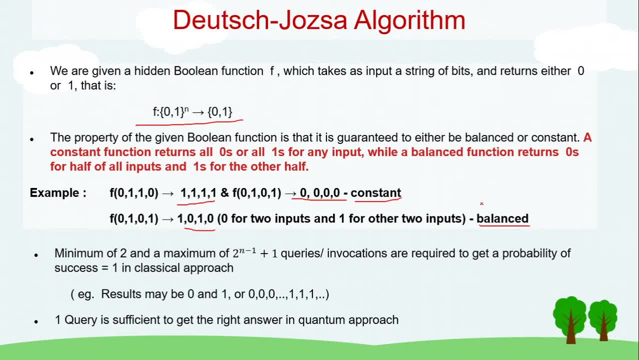 whether it's a constant or balanced, but how many times you have to make the query or how many times you will invoke the function? minimum two. we have to do it right. suppose first time we get zero and second time we got one. we are very lucky that with minimum two queries we are able to. 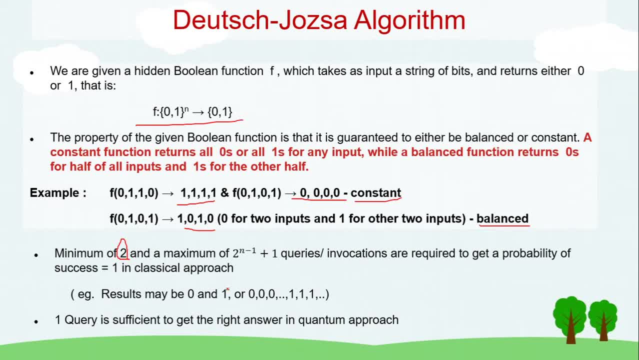 find out whether the function is constant or balanced. instead, if our luck is not good, let's take, let us assume, that we are given 10 bits first, five times i mean five inputs- it gave zero and then, at the sixth instant, it gave one. so what does it mean at the sixth instant or after making six times the? 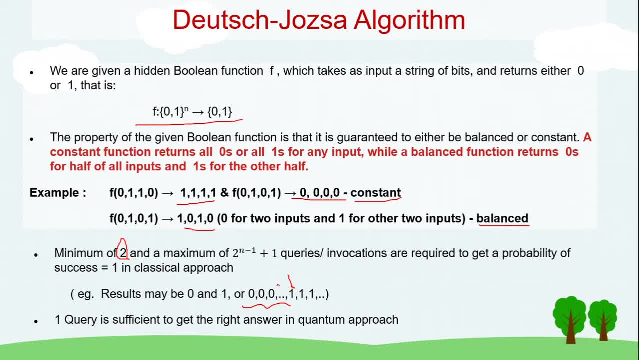 query, we were able to decide that i mean not design. we are able to confirm that the given function is a balanced one. so how did we get six, half of ten plus one? suppose we are given n bits so you have to make two power, n minus one plus one queries: is that clear? which is half plus one? 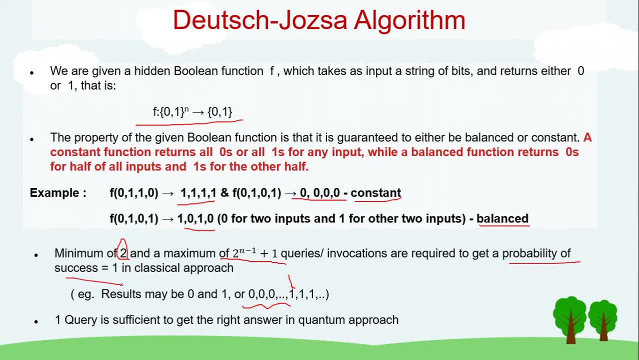 so then only you get the probability of success equal to one in a classical approach. now, if i make one query in a quantum approach and we get the right answer, will it not be wonderful if we can solve it, this first common riddle, if you fit the Wochen spin Clever way well. 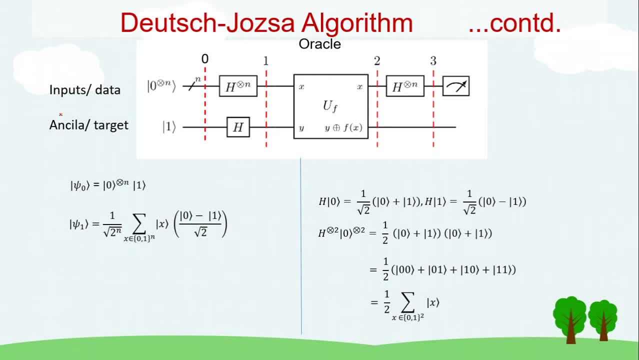 because if you divide by樂, you accept other solutions at a certain length of time. one mother where you have a gradient, even though- no, no, that is a coherent, simple algorithm. i mean the final answer. at the n-th number, third number, this problem comes first. 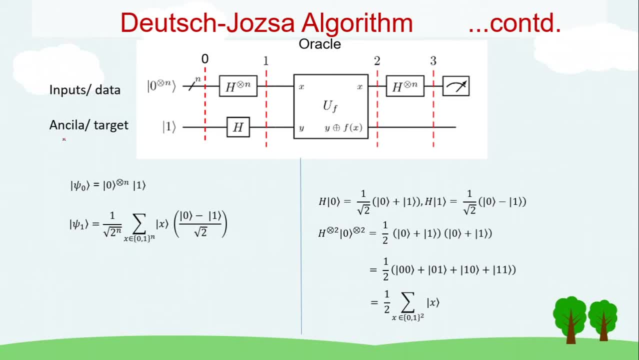 and that is in one state. so this is called ancilla or target. so, uh, ancilla, it comes like a substitute and use it for some time and then afterwards you don't care about that. so that's a special terminology we use and then we apply hadamard gate for all the qubits of then we call that: 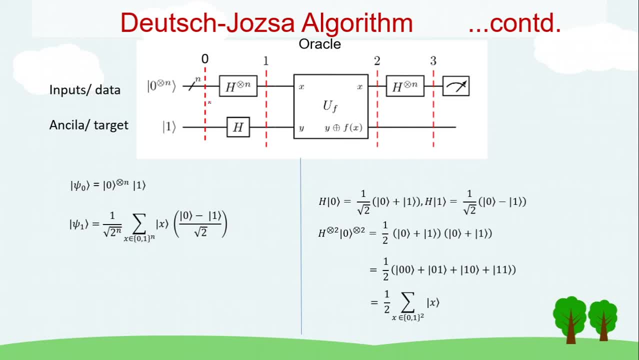 as a station one. so station zero is a initial state of the qubits. then we apply some gates, so here we get a station one, then we apply something called oracle. so what is oracle? so it's again a black box that contains a lot of operations. and then it it does something special. 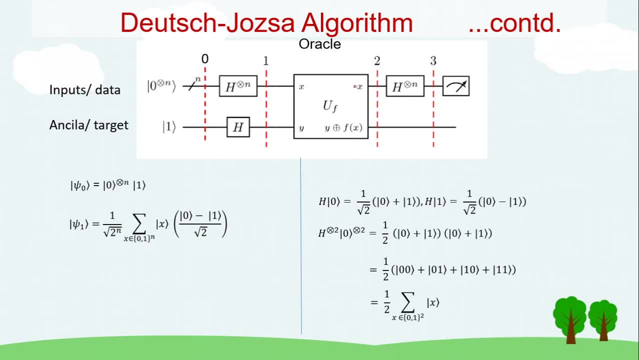 so it takes x and y here and then gives out x and y, some modulo f of x anyway. we'll see more details in the subsequent slides- and the output of oracle is station two. then we apply again hadamard gates on this set of qubits and then you get at this place. 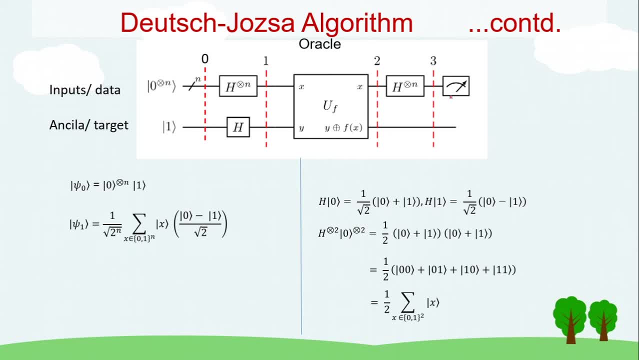 the. at station three, we make the measurement and decide on the result. okay, now let's start. so at station zero, the state of all qubits is given in the expression like this: so this is a new expression, but you don't have to worry. it says that i have n qubits in. 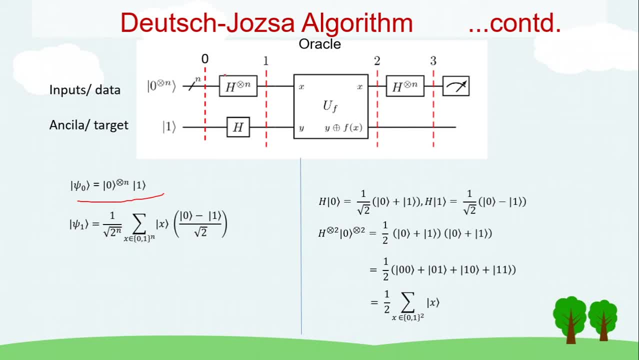 state zero. that's all okay, so it's anyway. that's what we want to start with. so no confusion. we leave it like this. this is just an expression. so then we need to apply hadamard gate. so, after applying hadamard gate, the result at this point, station one, the state of all qubits, is given like: 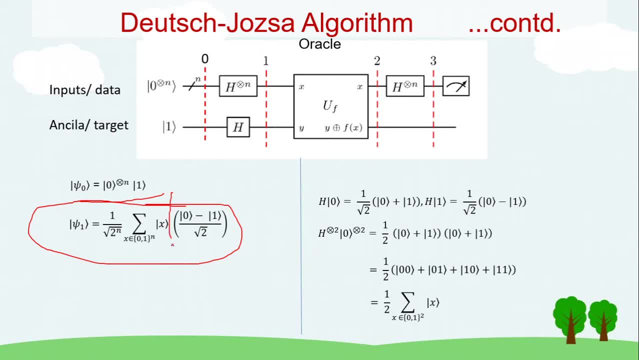 this. so this we are familiar, that is for one state, one. we know very well that hadamard will give this result. but what happened to the n qubits, which are, which were in state zero? so that is given by this expression. how did we get this expression? let's have a look at it on this side. so typically we 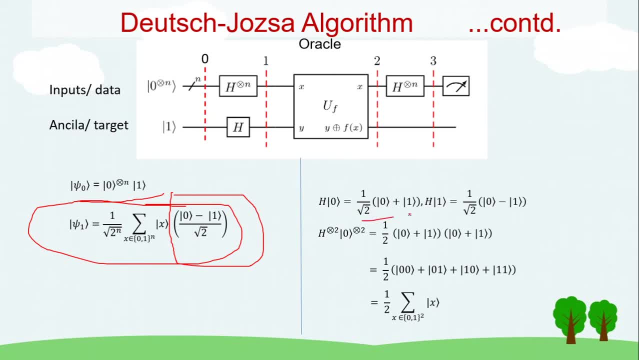 know that hadamard applied on state 0 is this one and state 1 is this one, so that this is the one we are having it here for this one. and if we apply hadamard gates on two qubits at state zero, what you have to do it, you have to do it twice: zero one into zero plus. 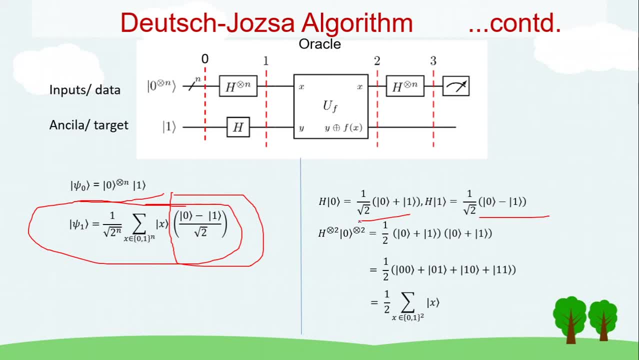 one right zero plus one into zero plus one and one by square root two will become half. and if you multiply further, if you simplify, zero, zero, zero, one, one, zero, one, one. this we have seen this right earlier. and for two qubits case, it's okay. we have four states, suppose. if it is three qubits, we'll. 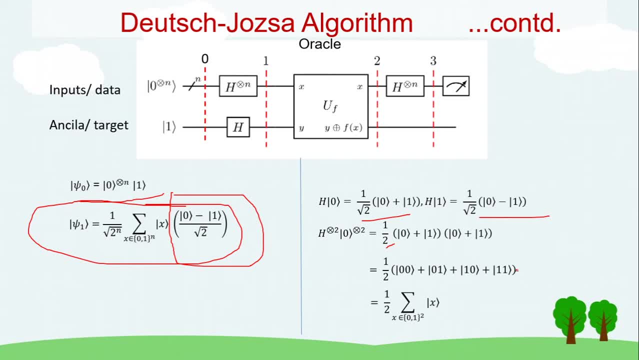 have eight states and for n qubits, oh, we have two power n states. so we don't want to handle such a large expression. instead we will say: it is x, where x represent all the combinations of the given number of qubits. so in this case it is: 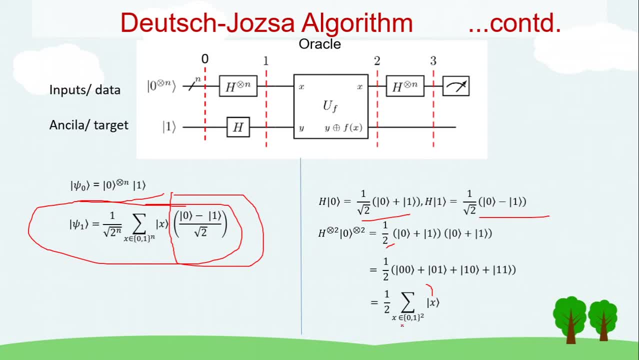 three qubits and we have four states and for n qubits we have two power n states. so we don't want twice, i mean two qubits. so we have written like this: x is an element of a set of zero, one half twice, and this is the straight x. and if it is for n qubits, what you have to do is replace: 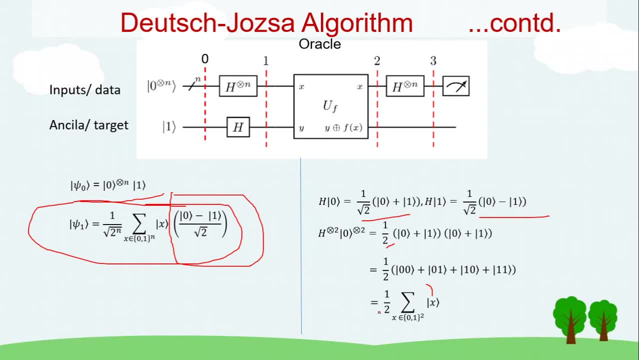 two with n. so this is nothing but in fact square root of two to the power of two. so right, so that will become two to the power of n, and this set value will become n. so this is what we have to do. so, after applying hadamard gate at station one, the state of qubits is given by this equation: 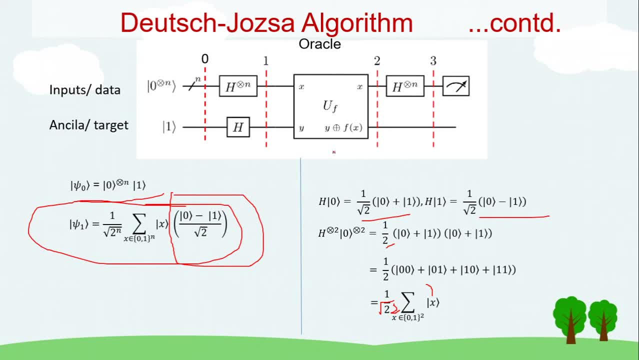 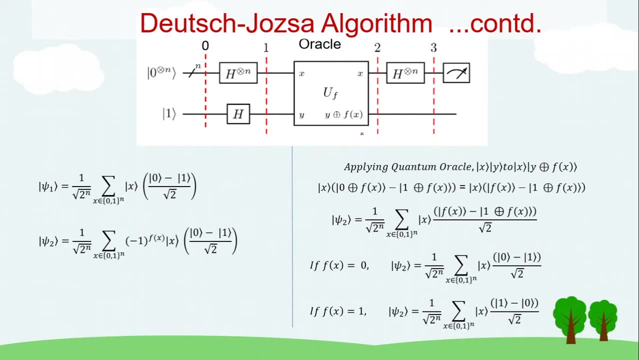 now we'll try to apply the magic oracle and see what happens. so this has come from the previous slide, no issue. and after applying this oracle, this is the value we are getting. so this remains same, nothing much. and other all other things are remaining same except this. 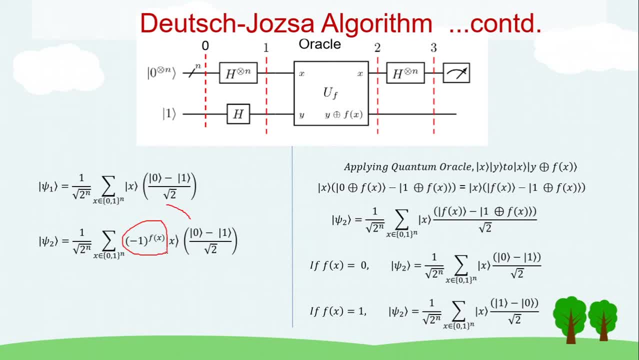 some scalar value has come into picture. so how did it happen? let's see what is the oracle? so we know that oracle does like this: takes x, y state and then give x and y, some model f of x state. so we need to apply. so x will not touch. so y state, we know y state, y state is nothing but. 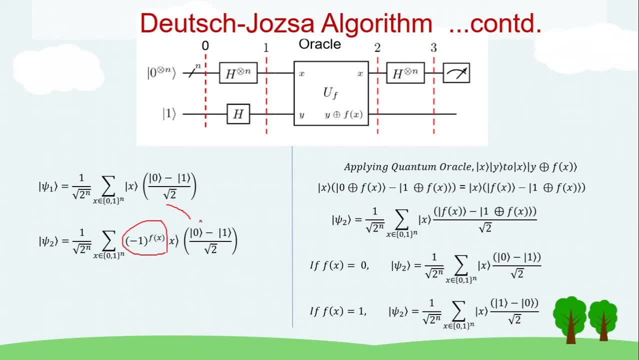 zero minus one state. so we have to say zero, some model f of x, one, some model f of x, so zero, some model f of x. we know that it is nothing but f of x itself. the zero doesn't affect the value, the output, whereas one plus one, some model f of x, we don't. 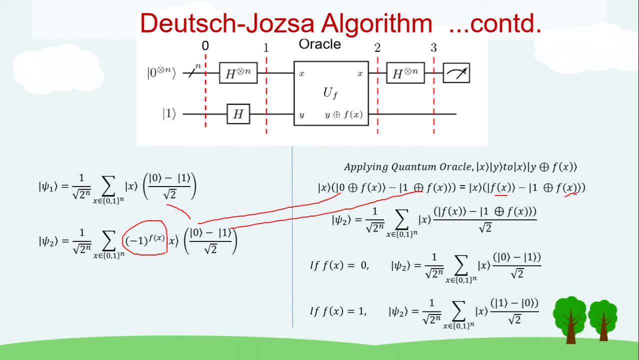 know what is the outcome, because it depends on the f of x value. if it is zero, then it becomes one, if it is one, then it becomes zero. so that is what is written here. so for again, for psi, two can be expressed as f of x minus one, some model f of x. so and now let us 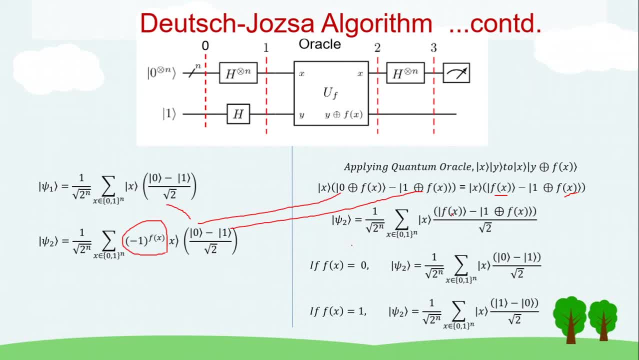 understand what happens if f of x is zero or one. if f of x is zero, what happens? so this will become zero and one. some model of zero is nothing but one. so we have got zero minus one by square root of two. if f of x is one, what happens? so f of x is one, so we have put one and here this: 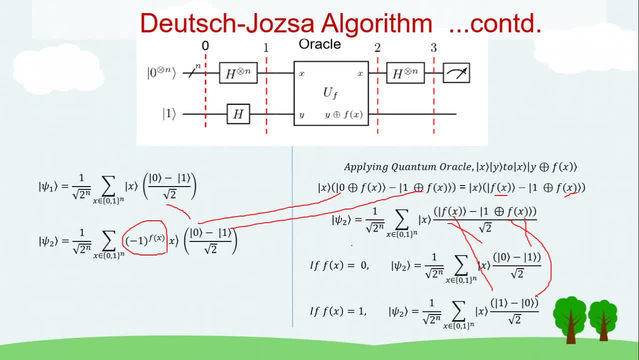 will become one, some model of one which is nothing but zero. we have seen it earlier, so interesting things are there here. so if f of x is zero- this is, i mean this expression- is zero minus one, and if it is one, it is one minus zero. can you write it in a better way, in simple term? so that is what has 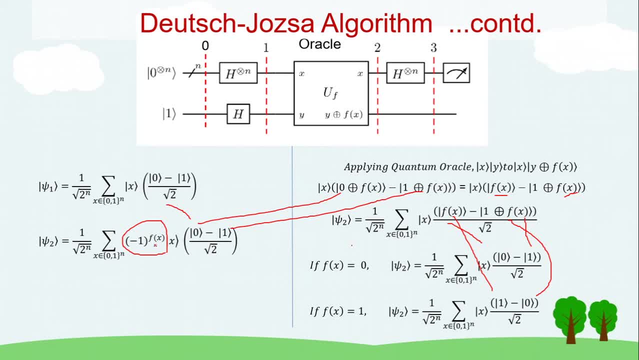 been done here, minus one to the power of f of x. i mean, these guys are great. so which says that if f of x is zero, it will be like this: if it is f of x one, then the signs get interchanged. very good, okay, now we'll move to station three. and how do we reach station three? by applying hadamard gate. 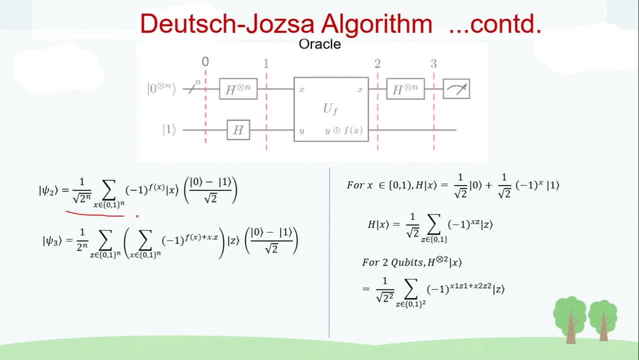 again n number of times. so state two: it says: come from the previous slide, no, nothing to worry. state station three: what has happened? so you will see something here, nothing much. this side, something has happened extra, and then you have some additional terms coming into picture. so let's see how we got again, because we 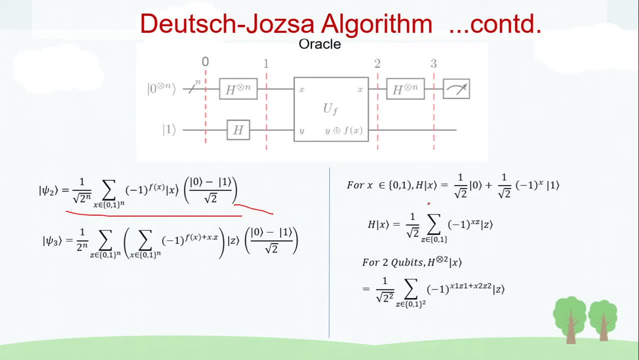 are going to apply hadamard, but this time we'll express our market in a slightly different way. we know always, whether you apply hadamard on zero or one, the first term doesn't get changed, only the second term. it will become plus or minus, depending on whether x is zero or one. so that is what is written, like this: if it is zero, then it is. 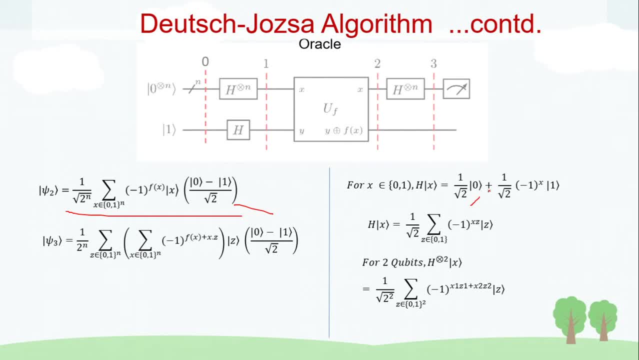 plus. if it is one, it will become minus. so why did we do that? it has got some advantages. we'll look at that. so this can be simplified now like this: if hadamard is applied on x, instead of writing two terms, I'm going to write it. 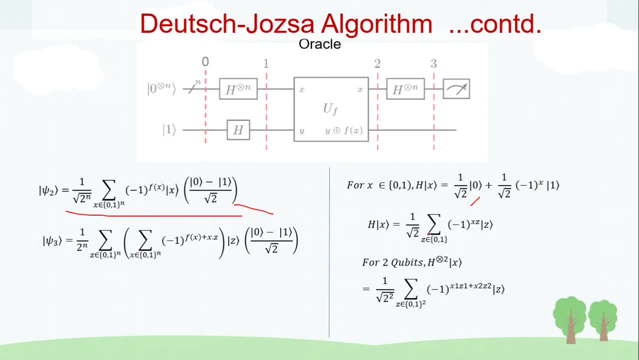 in a single term, right with a sigma in it. so let's say x is 0 at that time. what happens? so? first, this will leave it for time being. so I'll put minus 1 and the z can be 0 or 1. okay, so first case will. 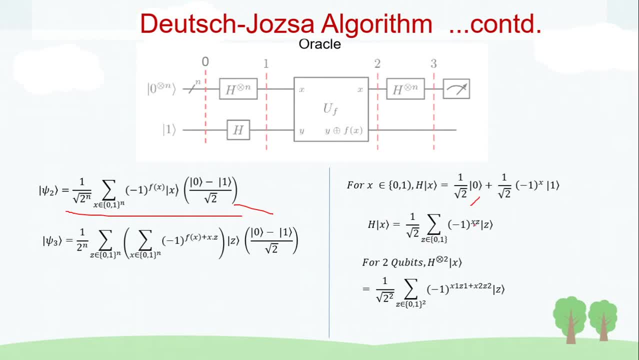 take X is 0, Z is 0, x is 0, z is 0, x is 0, z is 0 minus 1 to the power of 0. then I'll write it back: 0, z is 0, minus 1 to the power of 0 is 1 and z is 0. So this is nothing but 0 state. 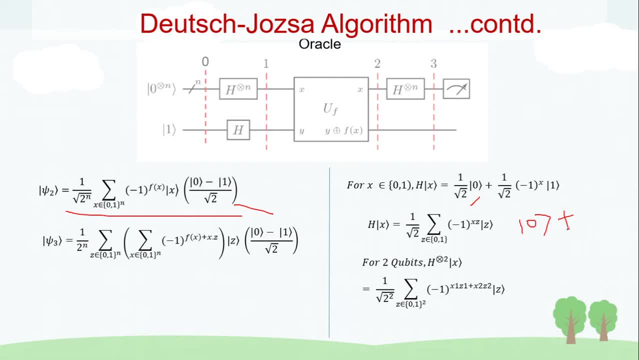 Now, because of sum, we will put the plus sign. Now again, x is 0, but z is 1. So 1 into 0 is 0, minus 1 to the power of 0 is 1. So and z is 1.. 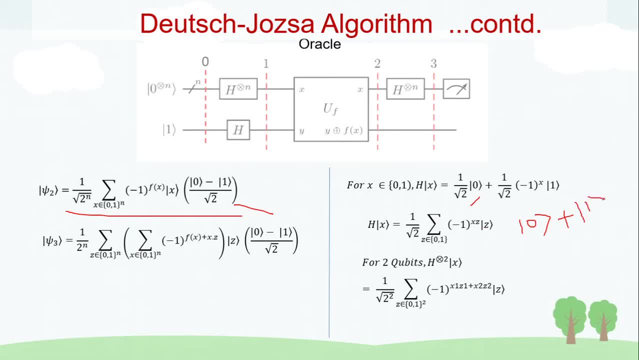 Now clear, And if x is 1, you will see minus sign. here I mean that you can do it as a homework for you. Clear. So same Hadamard gate. we are trying to put it in a simple way. I mean sorry, not in simple way, maybe a complicated, but very useful way. 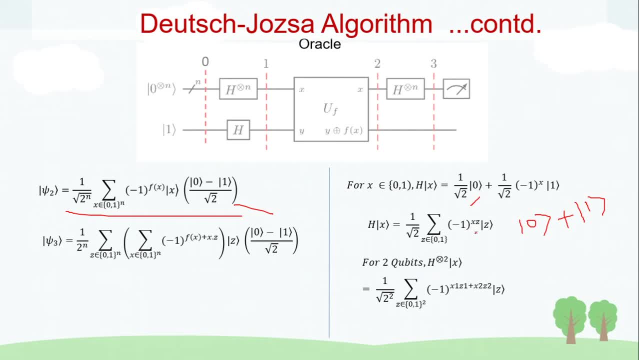 So for 2 qubits case, what happened? So this will be doing it twice. So it will get added like this: x1, z1 plus x2, z2.. And then you will be doing twice. So that is why this has become twice. 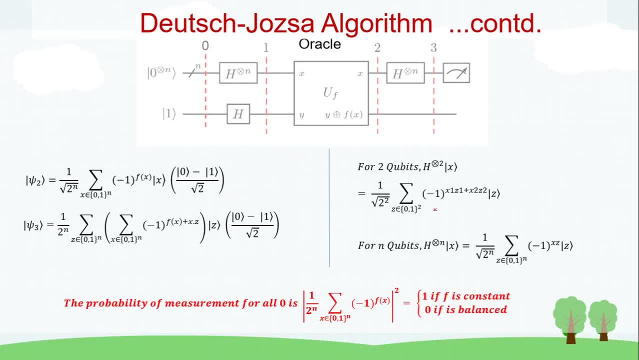 Okay, Now what happens if it is n times? So I just copied from the previous slide. So n times again. whenever, wherever 2 is there, you replace it with n, Here 1, n, here 1, n And this one. what we are doing is, instead of writing x1, z1 plus x2, z2,. 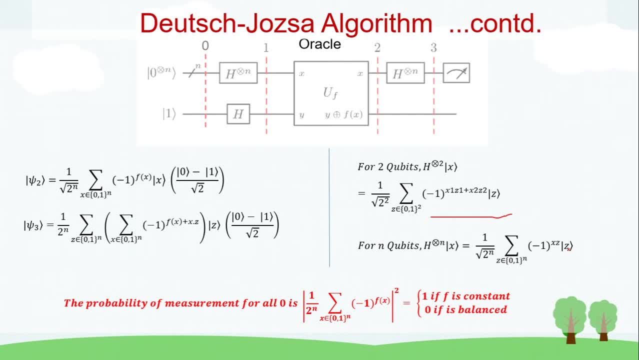 like this: up to xn, zn, you have to enter right. Instead we will say xz, That's all, Which means nothing but x1, z1 plus x2, z2.. So this expression has become simpler, So. 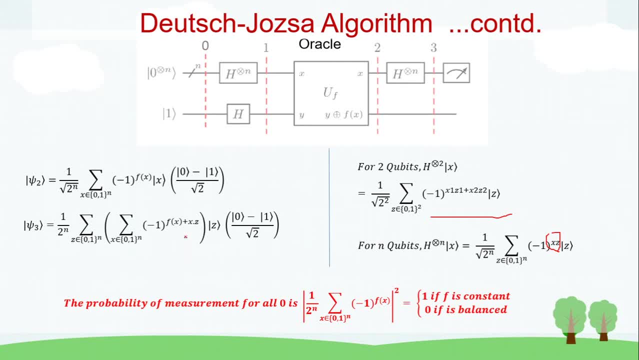 that is what has gone into this place here. So now we have got two summation, sorry, and actually we have got an answer already how it's not direct. one say, in a conventional way, we pass all the qubits. look at the result. 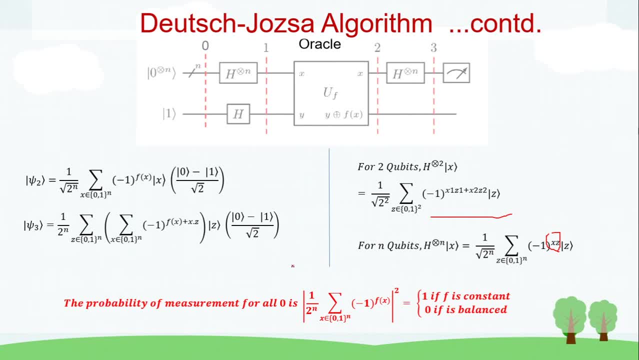 then you say based on the results, whereas here we are trying to interpret the results in a slightly different way. so please be watchful. so what we are saying is the probability of measuring all qubits at zero state is given by the magnitude of this expression. so you take the magnitude. so for all zeros. so this: 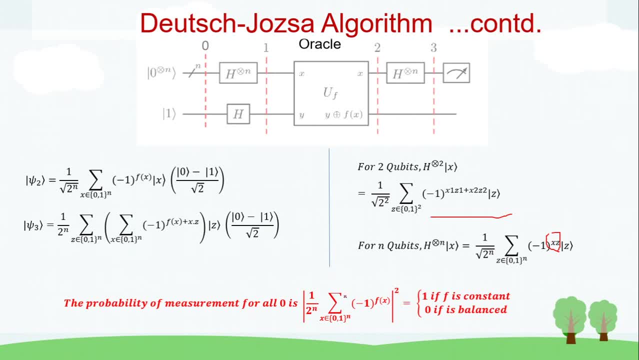 will go off and you will have 1 by 2 power n sigma minus 1 to the power of 1. so this will go off and you will have 1 by 2 power n sigma minus 1 to the power of f of X magnitude square. now let's look at the two possibilities. if F is, 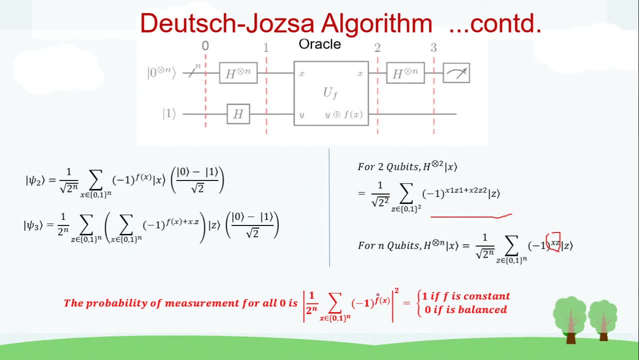 constant. a given Boolean function is constant, what happens? we will have 1 or 0. so let us put first the case minus 1: 1 to the power of 1, plus minus 1 to the power of n. 2 to the power of n. 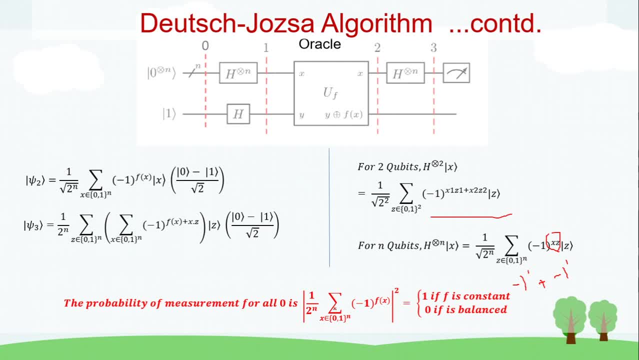 so, since we are taking the absolute value, so you will have 2. like this, you will get n number of times and finally the net result is you get 1 if F is constant- constant. when f is constant with this one value, same thing will happen when it is 0. so 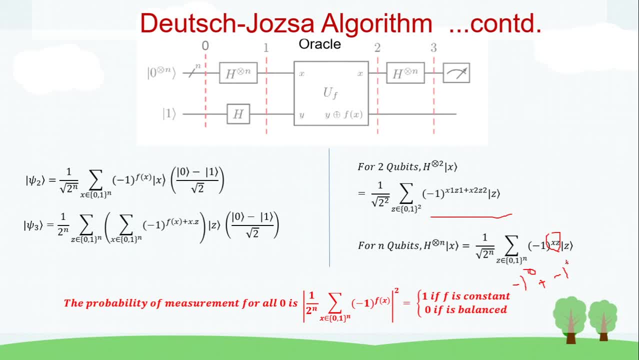 this will become 0, this will become 0. so what? you will get 1. so you will get 1 plus 1, like this n times. so again same, you will get 1. that means if, if f is constant- I will get all qubits here- 0. let us say what happens if it is. 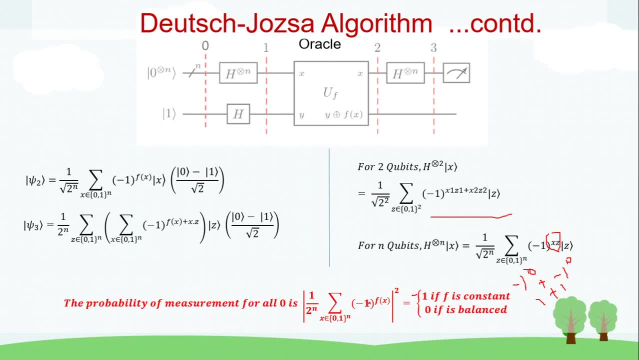 balanced if f is balanced. so what happens? so you will get once 0 and another time 1, which means you will get minus 1 plus 1, and that will get cancelled. you may get 1 and that will get cancelled. you may get 1 and that will get cancelled. you may get. 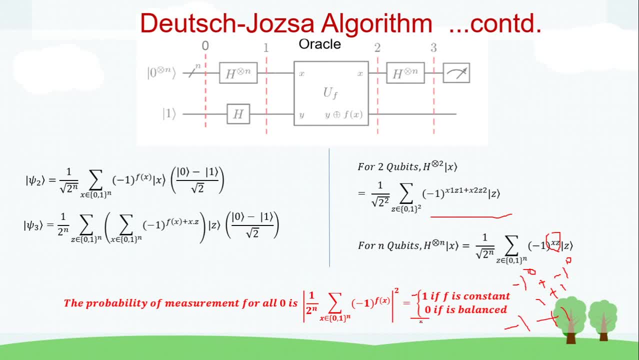 and finally you will end up in 0, clear. so this will happen: minus 1 plus 1, minus 1 plus 1, minus 1 plus 1, like that it will keep happening and at the end of the day you will get 0, the value for this expression, if f is balanced. so at: 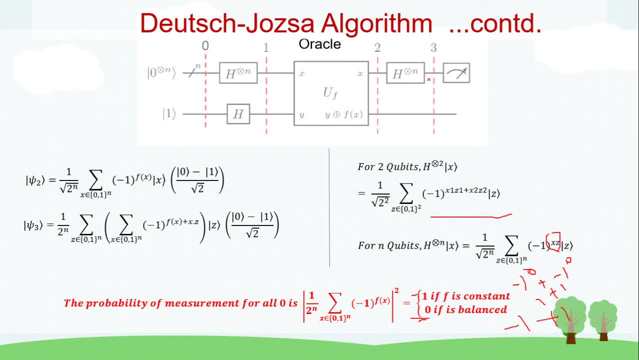 that time what happens? so the probability of getting all zeros at this location is 0, which means you will get all ones. so if I measure all ones here, I know the given function is balanced. so that is what. again, we will prove it in a quantum computer or simulator, but before that we will thank. 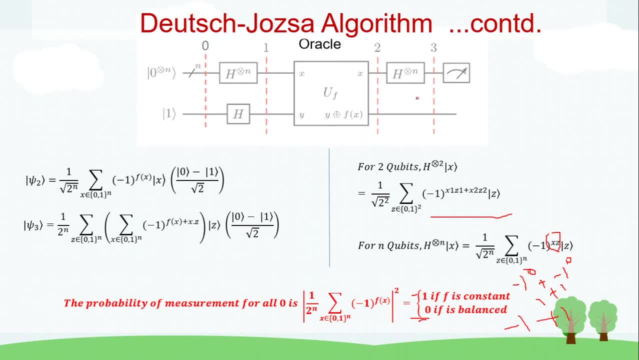 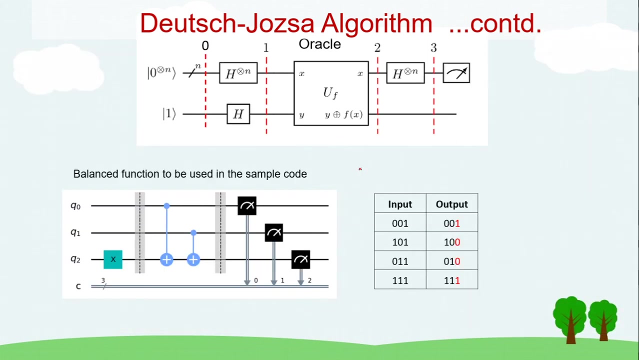 DJ that with one pass they are able to determine the given function is a constant or balance, a lot of magical things happen. possibly you will understand more of you. I mean, try to do each and every operation in more detail the way. so we are going to program this in a quantum computer at that time we need to have one.